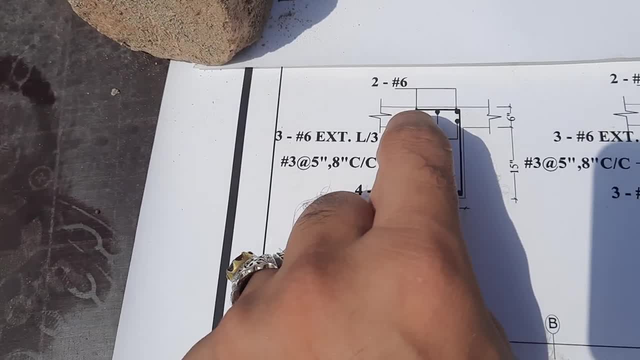 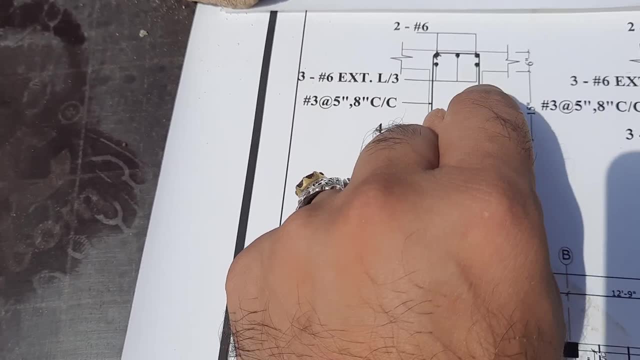 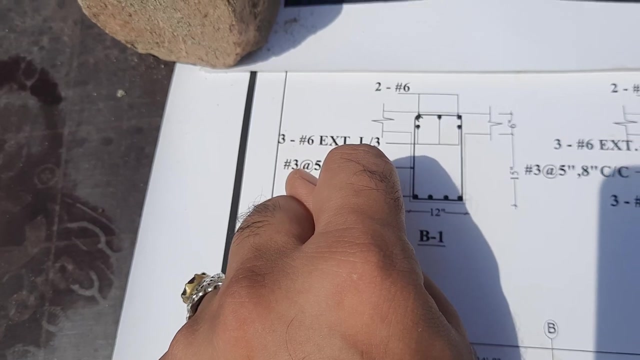 top. okay, one is this one and this is the other one. dia is six number, two numbers. we have also guys. you can see we have also two, uh, three, sir, to our sidebars. one is at the middle, okay, so three numbers. dia is six number. okay, exact l by three at the distance of l by three. we have this one, okay. 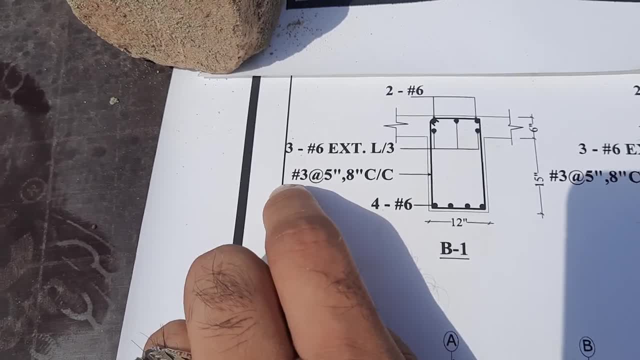 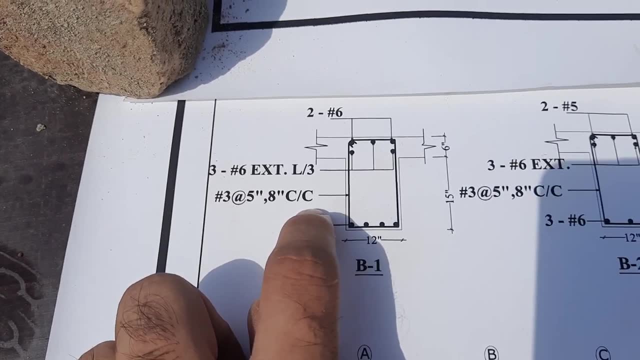 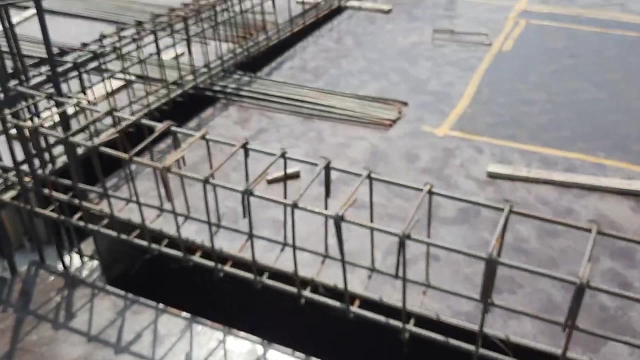 so next, guys, you can see, see the stirrups and the dia here. the dia is three number at the spacing of from five to eight inches center to center distance between each stirrup. okay, so, guys, this is red section and this is its layout plan. now let me show you, practically okay, as you can see, this is b1 from this column. 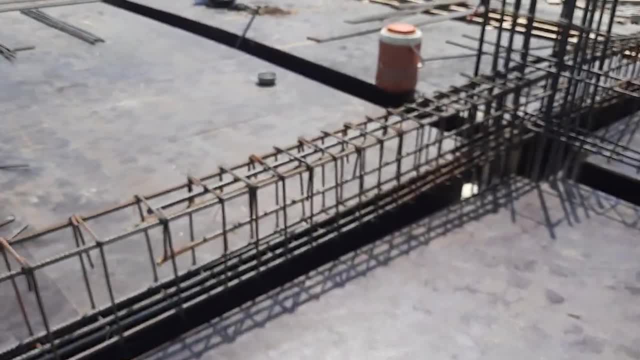 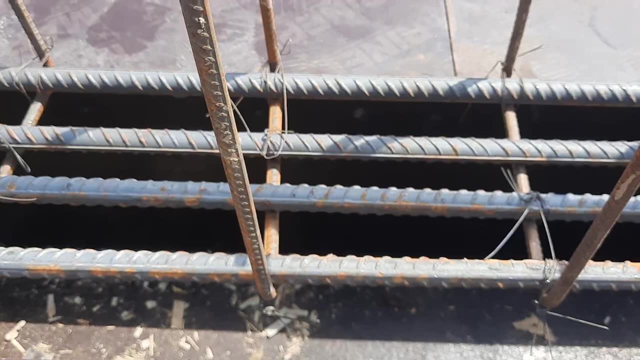 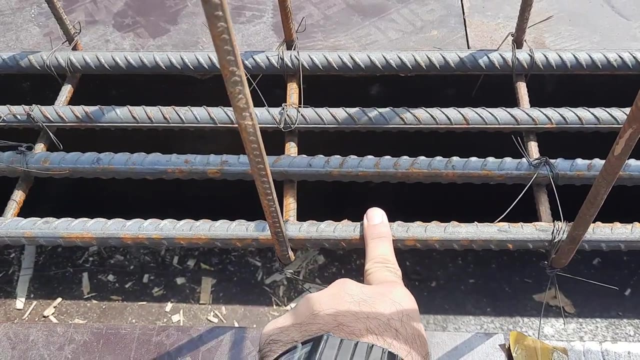 center to this column center, the length is 20 feet and 9 inches. okay, so here, guys, you can see clearly. we have four numbers, as i show you in the drawing already. so we have four numbers, we have six number of steel rod, four numbers of steel rods and bottom portion, and two numbers and upper portion, as you. 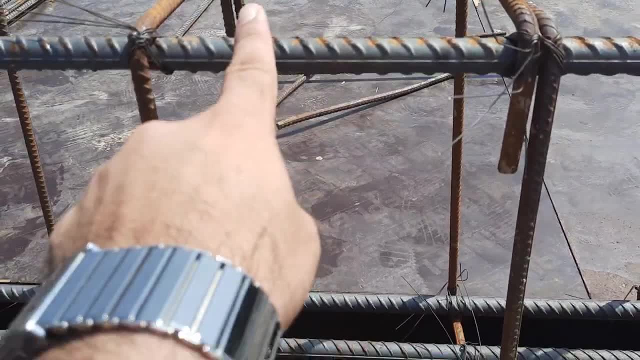 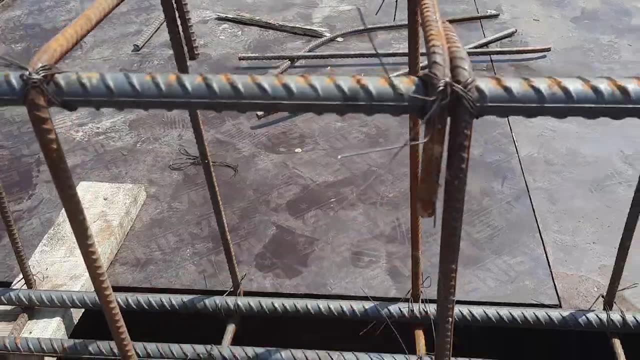 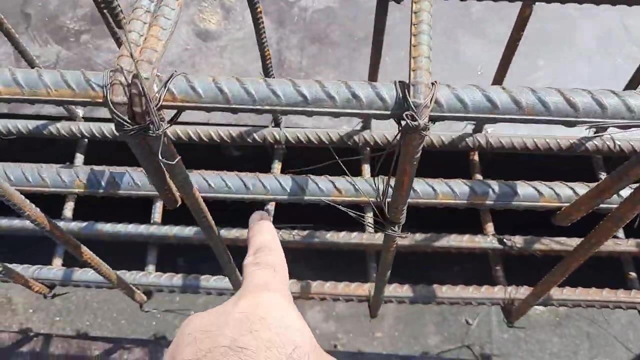 can see clearly. okay, the dia is six number also here. as you can see, the depth is 15 inches. width is 12 inches without slip, rcc, slip. next guys. let me show you for the other section. as you can see, we have the middle bar is the other one, and these are two side bars at the distance of l by three, as i show you in the drawing. 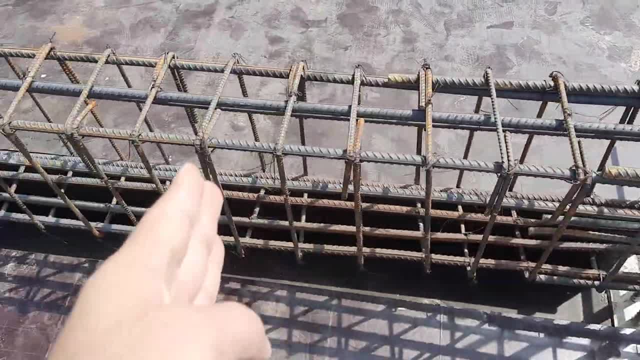 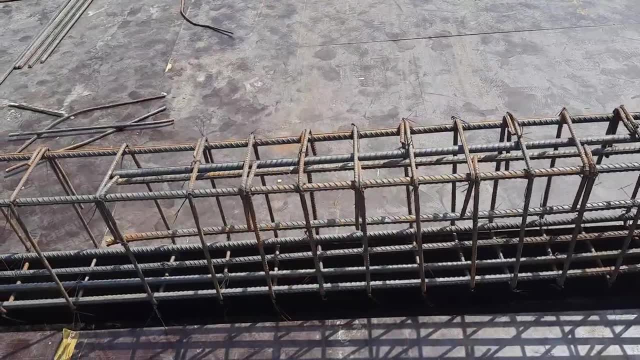 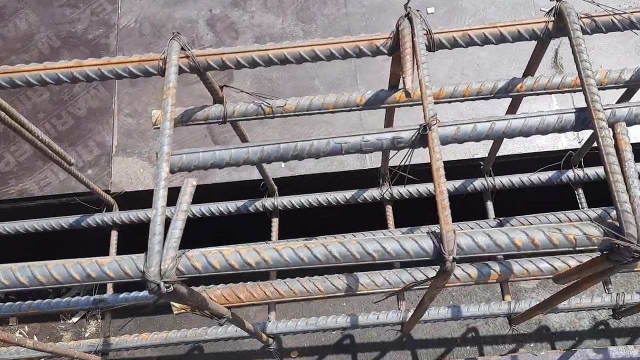 already. okay. so this is from this center to l by four, l by three- sorry, l is the spin between these two columns- and l by three. so total length divided by three. so here we have three steel rods, two are side bars and this is the other bar. so we have three numbers and the dia is six number. okay, 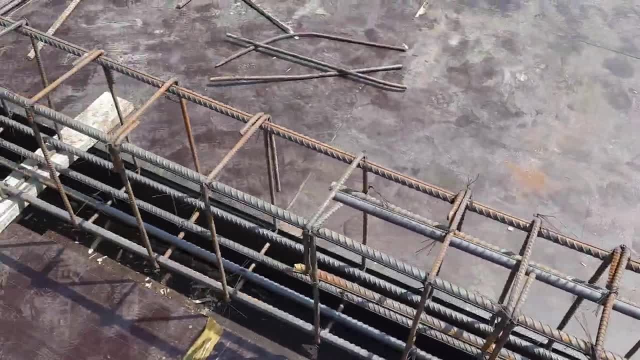 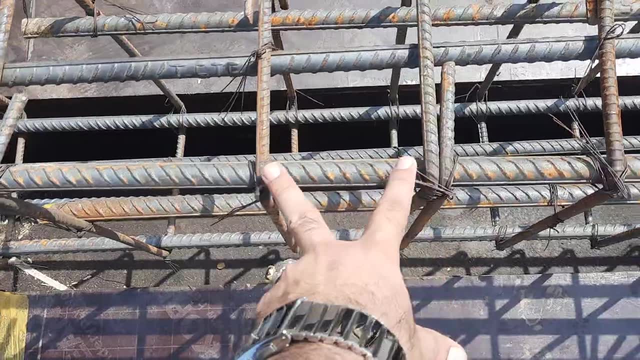 now let me guide you for its stirrups details, guys, the stirrup spacing. you can see this is eight inches, after l by three, but at the distance of l by three, guys, you can see clearly this is five inches. so five inches and eight inches. so these are the 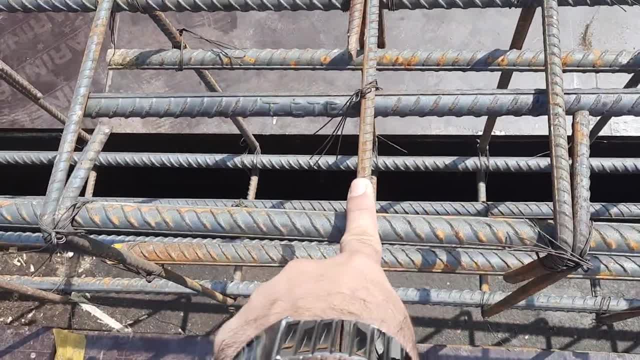 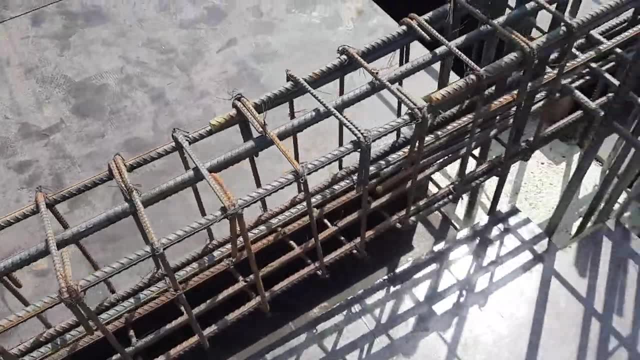 spacing. the dia of uh stirrup is here, three number three, number bar guys you can see- and the spacing is from five to eight inches. so here this is l by three, this is the column center. at the distance of l by three we have three steel rods. again you can see. the distance between these two columns is 8 inches. 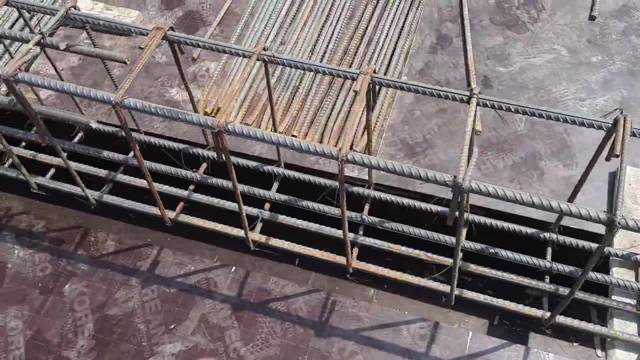 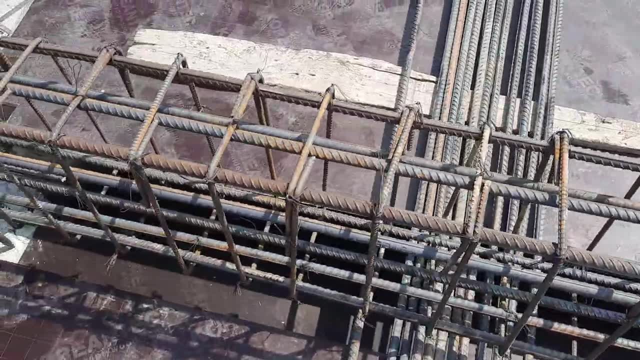 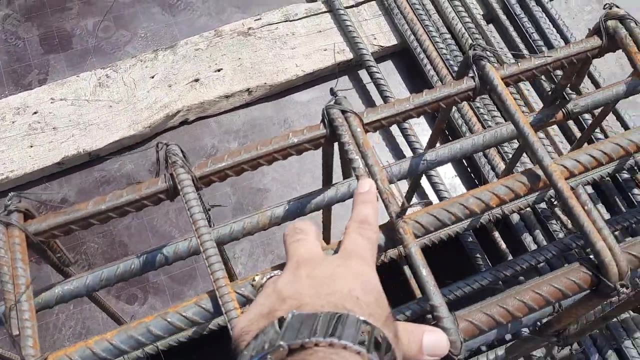 you can't see any extra steel rods, okay, and you can see the spacing is eight inches on this side. you can see clearly this is five inches, okay. so one thing is very important: they didn't provide the hooks on 135 degrees, where it should be provide on 135 degree, not on 90 degree. so they 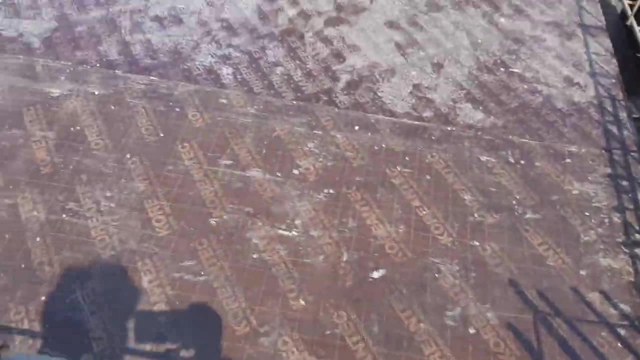 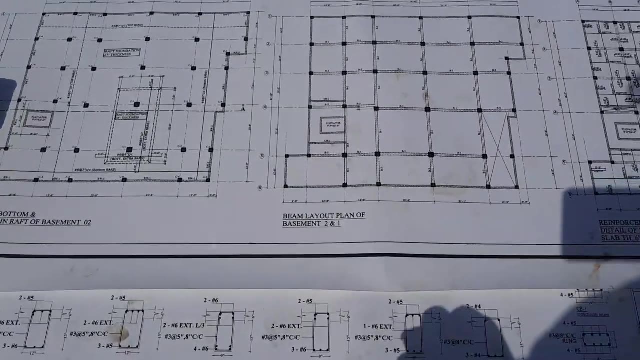 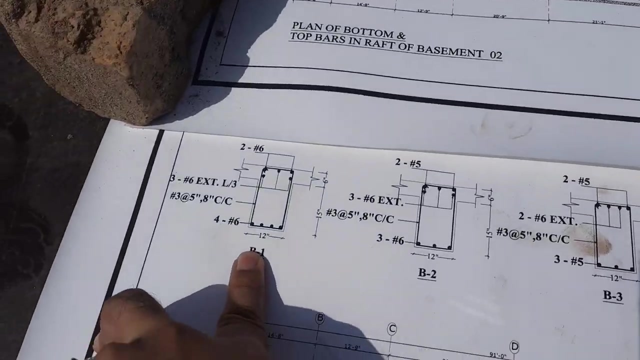 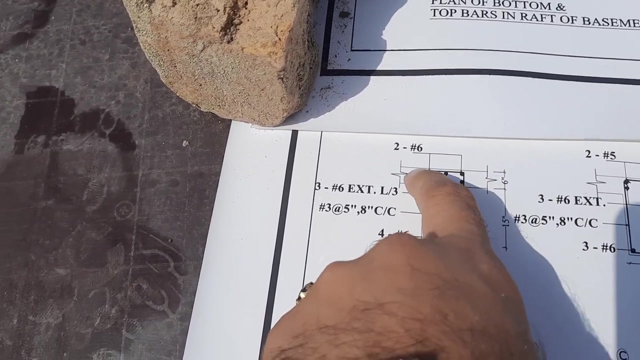 bend it on the 90 degree. so let me show you the drawing again. as you can see, this is b1- okay to 20 feet and 9 inches, okay, b1 section. and you can see a section b1 as I show you. they are practically four numbers we have at the bottom three. at the top two are sidebars and three one. 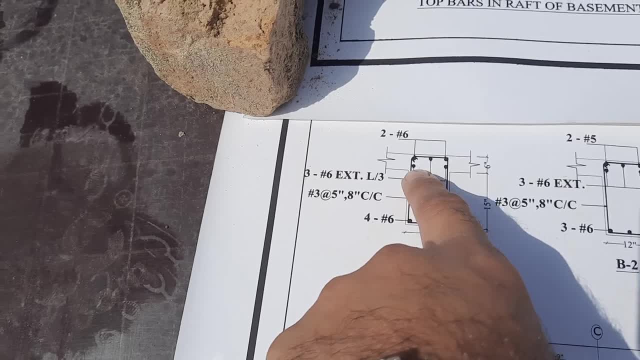 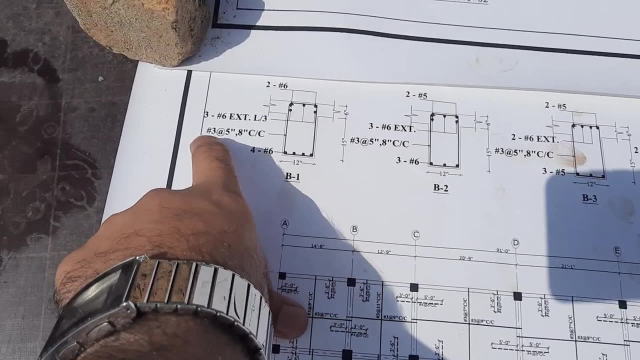 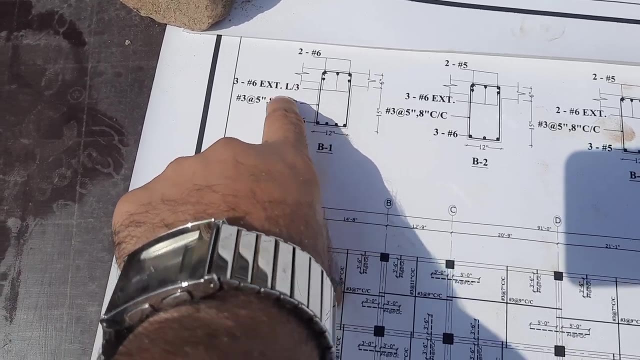 is the middle bar in upper portion to our sidebar. see at the distance of L by three. guys, you can see. at the distance of L by three. okay, you can see three number bar at the rate from five inches to eight inches, five numbers at the distance of L by three and eight inches after L by three. okay, you can see. these are the other sections. 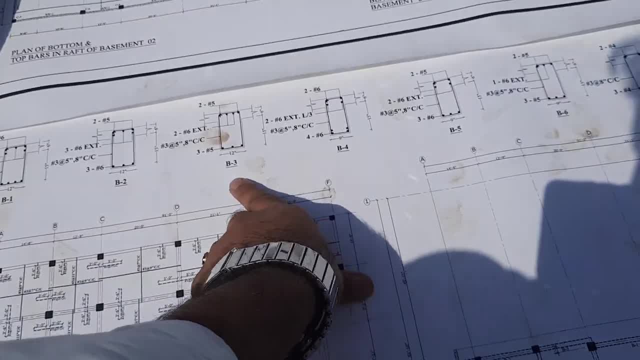 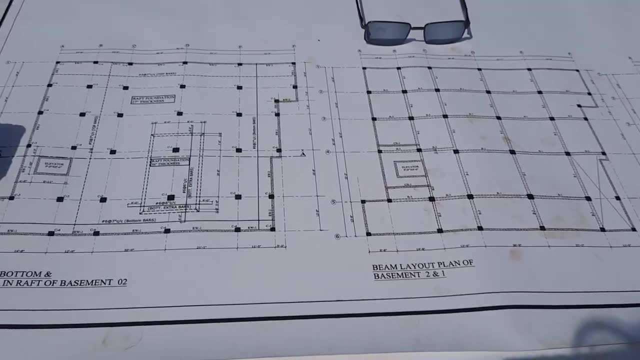 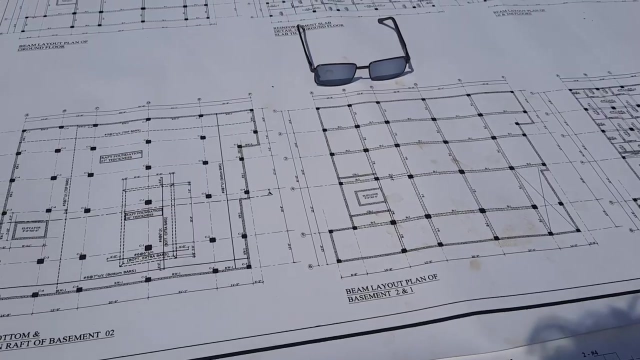 for the and be true. okay, before b3, b5. we have a lot of beams here and from this drawing you can get those are very important to know about how to read the drawing. so reading drawing is very important before starting the construction of steel reinforcement. so therefore I'm telling 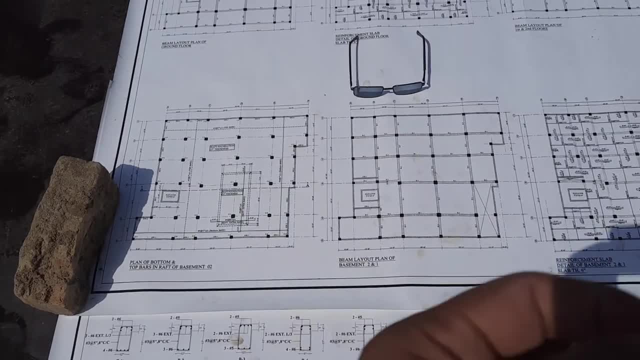 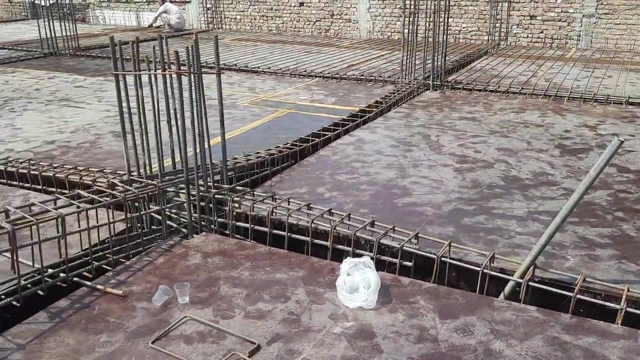 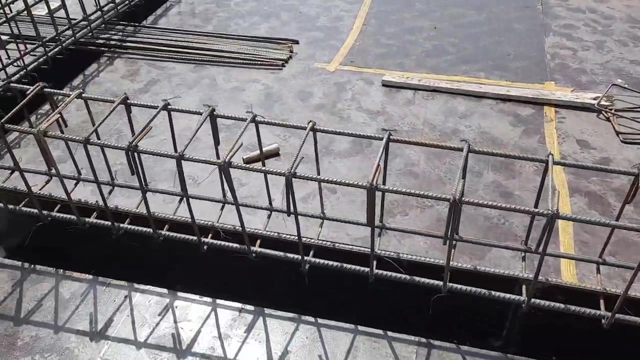 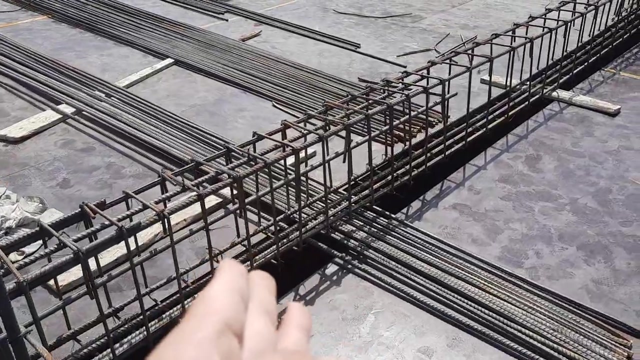 you if you are working on a construction site. so you should remember. you should remember how to read the drawing- okay, structural drawing or architectural drawing- and then you are able to see the layout after layout planning. so steel reinforcement. everything we can get from this is: you can see clearly. so these are steel reinforcements. so this is b1. okay, 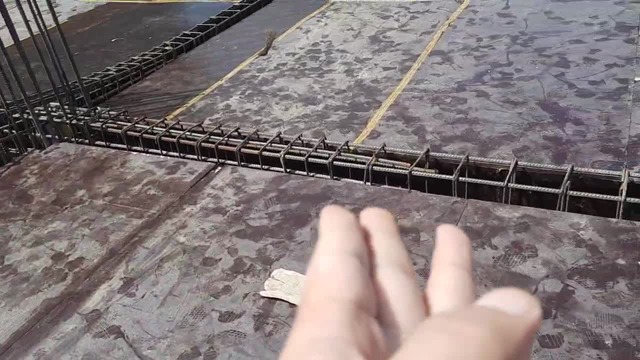 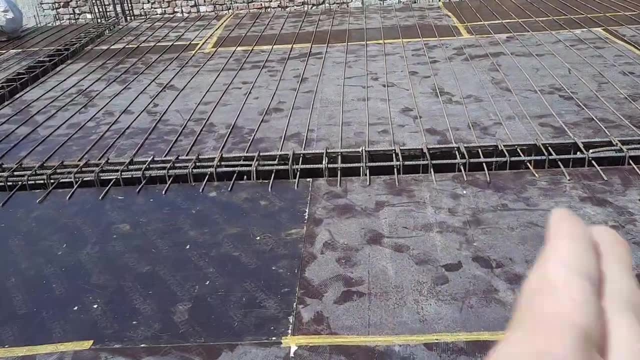 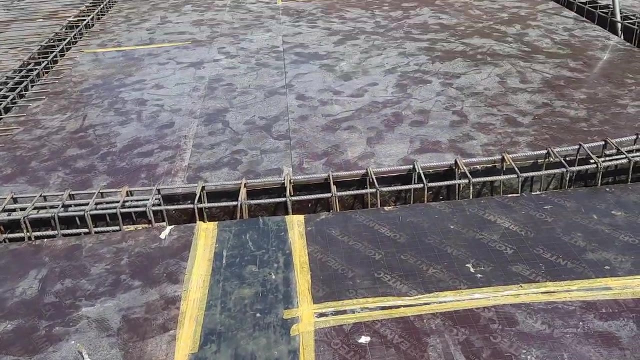 this is b1 and this is also the other b1. okay, beam number one. there is also b1, okay, so you can see the shutting. okay, the giants are closed by a plastic tape. so this is very important and these are technical terms which I'm showing you inedly. we are done, OK, in this video. in this video, this one is that we just get ready and we are complete and that be careful. contact with your sorts is a joint, uh, that sometimes data isuca, surface, whoa, but so its a joint. ok, I need to do a quick analysis of what only you牛 is loosing here to add some detail. okay, not just that. we can be, excuse me, with your 14, and this is what we need. is that necessarily reduce this, this huh, this one, right now, after. 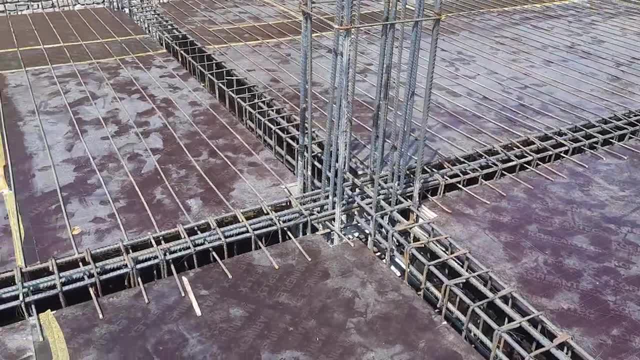 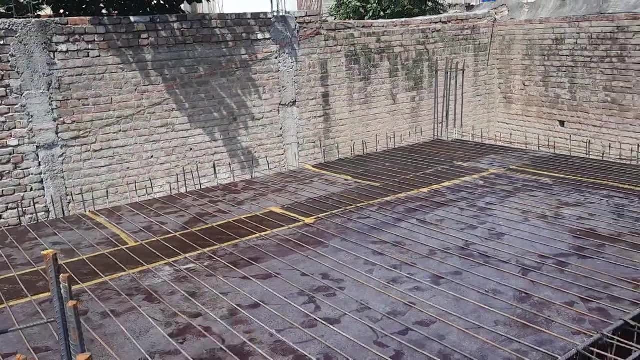 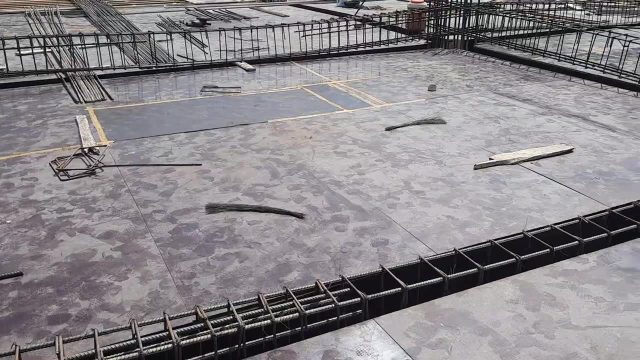 so this is very helpful for you people. as you can see, these are the other beams which is be true there. they will provide the beam that is b2, this one is b2, okay, and b1, b2, b3, b4, b5 each beam steel. 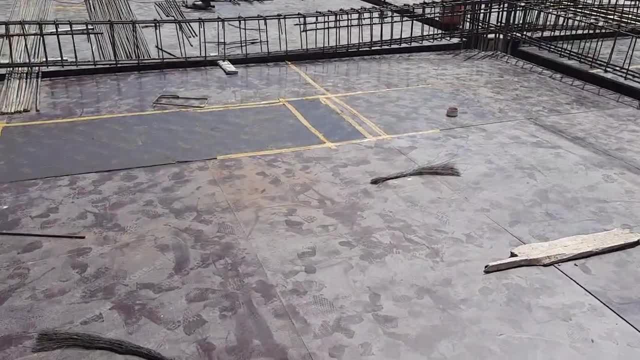 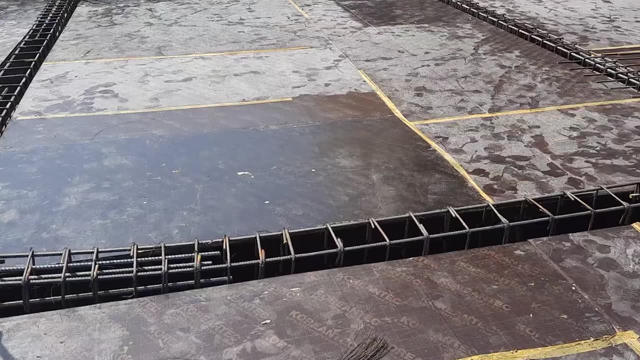 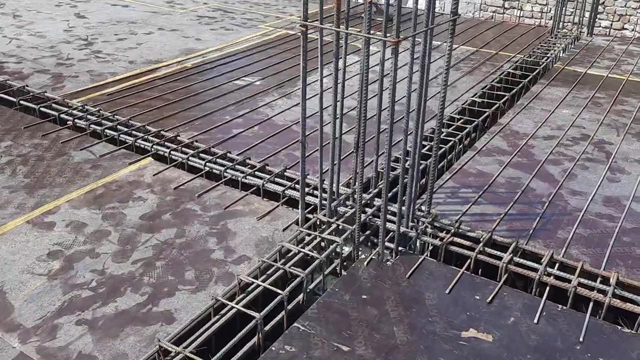 reinforcements are changed from each other according to structure load, according to the spacing, according to column size, according to a lot of things we have on the construction side. okay, so this is very helpful to know about this. as you can see, this is the column which is 24 by. 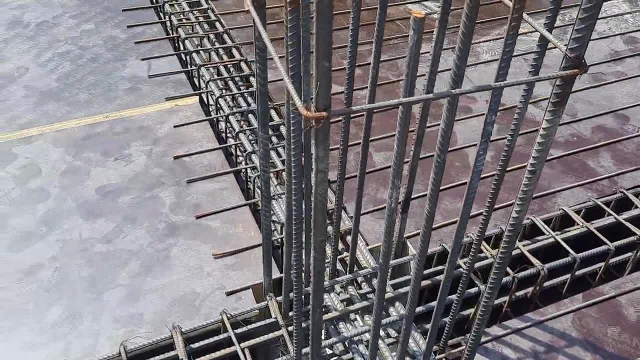 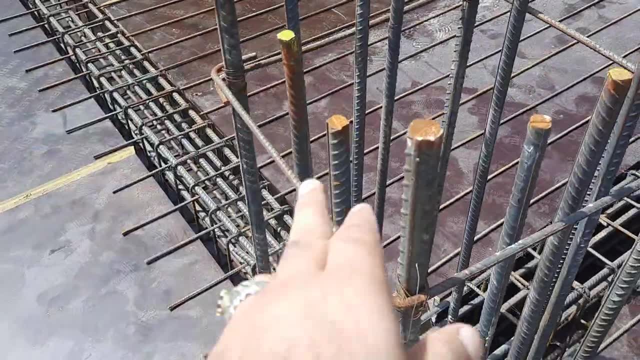 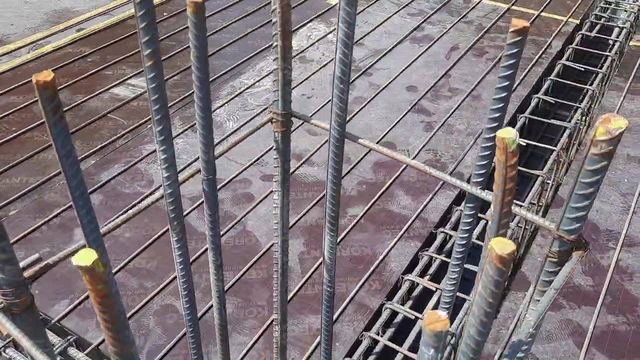 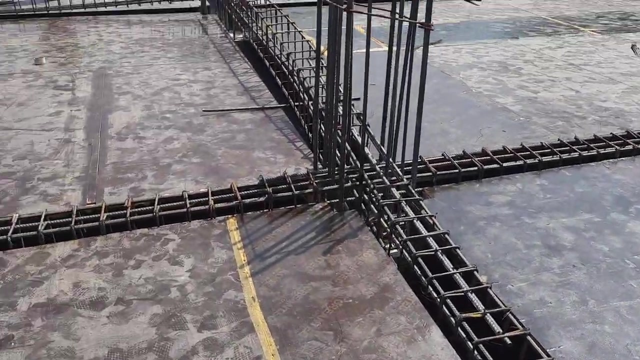 24 inches with concrete cover. you can see the steel reinforcement here we have 12 numbers of steel rods. okay, you can see this is 25 mm F number bar and you can see here 16 mm, 20 mm. okay, they used here 60-grade steel rods in this construction. 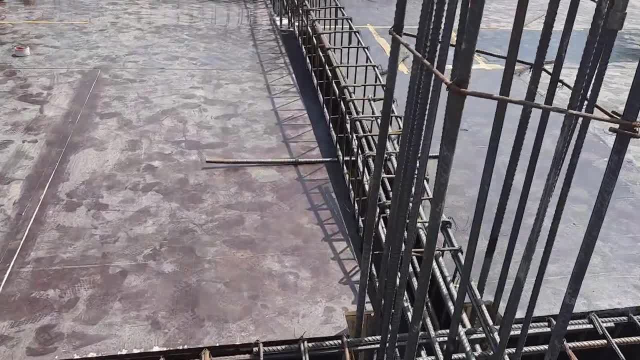 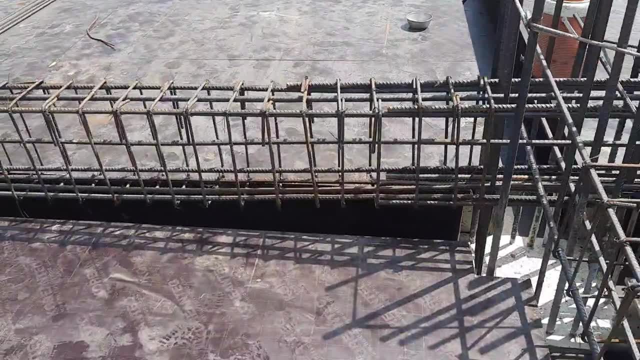 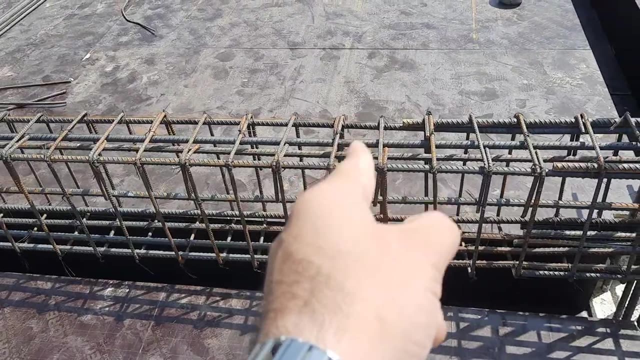 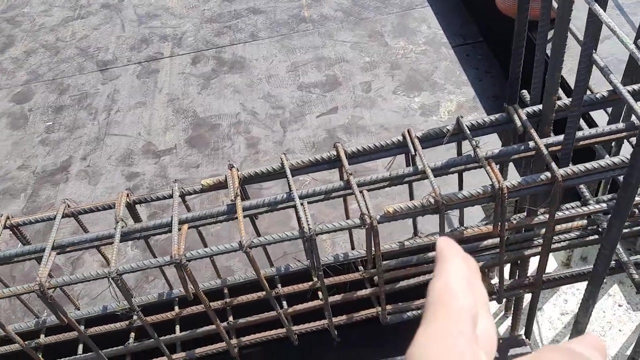 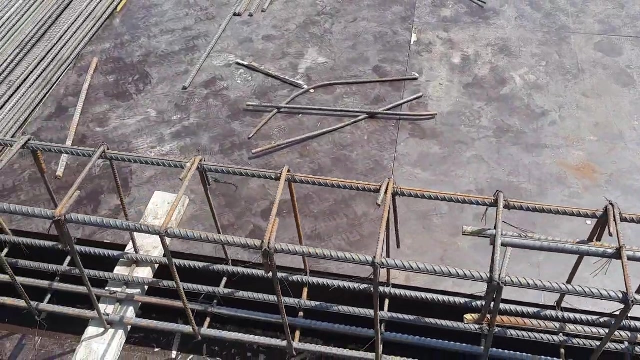 there is b2, which I have already discussed, for its size: bottom steel reinforcement. upper compression zone steel reinforcement stirrups details, extra steel rods and stirrups hooks. I already discussed the length of the stirrups. should not be less than 3 inches, it's okay, but the bend is provided on 90. 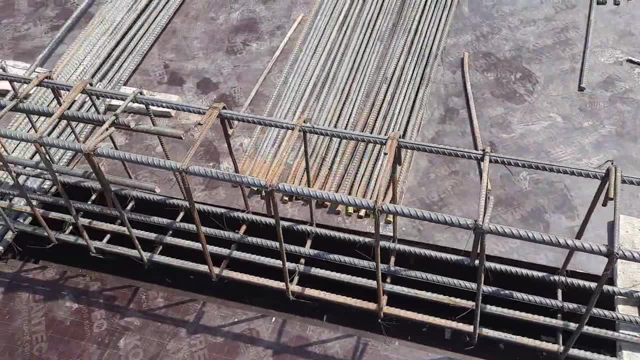 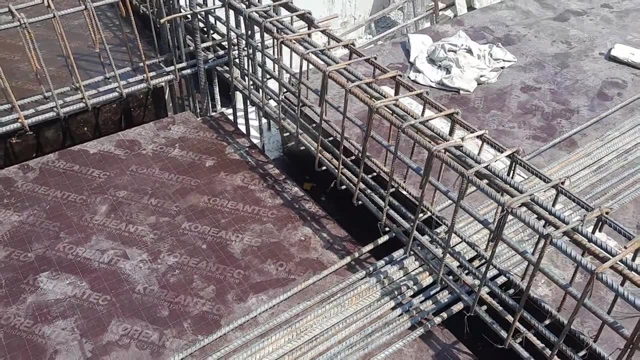 degree, but it should be provided on 135 degree. hope this short video can help you. if you have any question related this construction video so you can comment, I will try to reply your answer. thanks for watching. see you in next video. good bye.